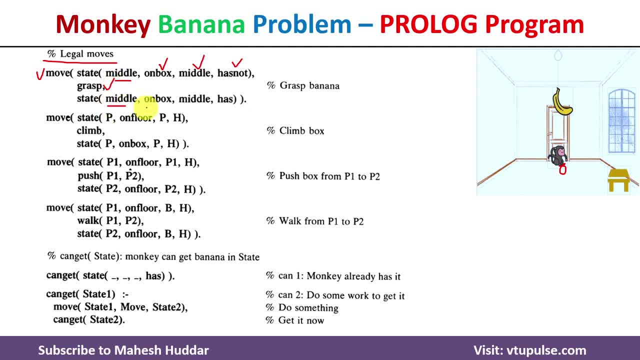 will be executed successfully and then monkey will be present at the middle, on the top of the box. and at the middle monkey will be present on the top of the box In the middle of the room. the box is present. Previously monkey was not having banana. Now 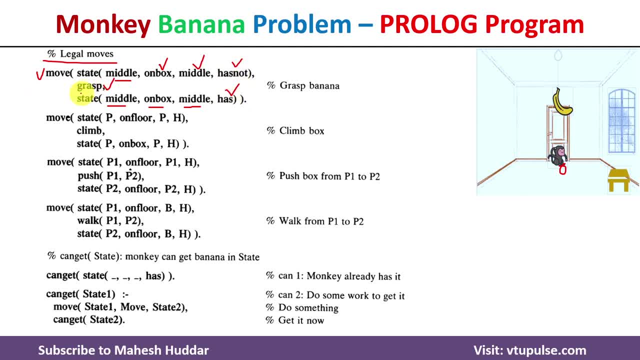 monkey is having banana over here. So this is how the grasp is executed. Coming back to the second move, that is, the clim, here Again to execute clim, I think I have already told you what are the different conditions. The monkey should be present on floor. Both monkey and the box should 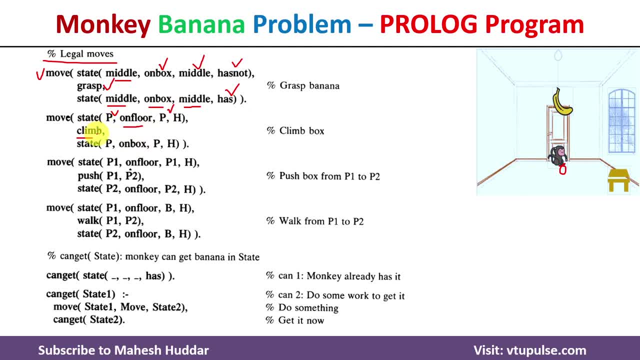 be present at the same position, that is P here. Once the clim is executed, the position of the monkey and the box will not change. It's a horizontal position. What will change? Monkey was present on floor Now it will be present on box here. That is the only thing will change here. 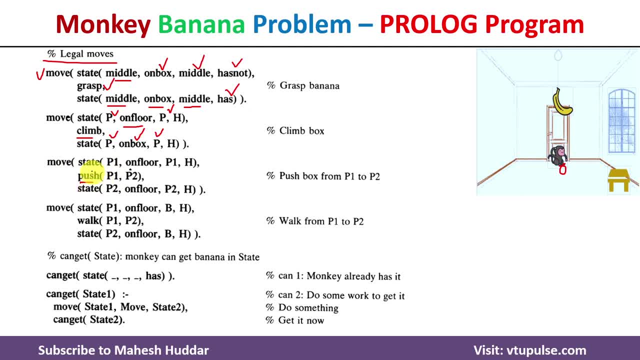 Coming back to the next move operation, that is push. here, Whenever we want to execute push successfully, both monkey and the box should be present at the same position. That's the reason. this is P1 here and this is also P1 here. We don't care about the monkey is having banana. 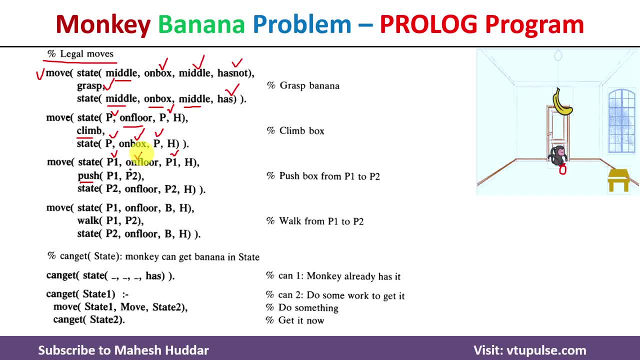 or it is not having banana. But what is? the one more condition is monkey should be present on the floor. Then only it can push the box from position P1 to position P2 here. That's the reason. the position of monkey will go to P2 here, from P1 to P2.. The box will go from P1 to P2 here Again. 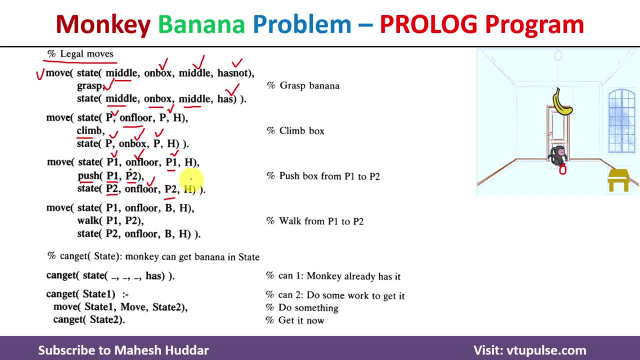 the monkey is present on the floor. only. We don't care about the last component here. This is how the push will be executed, or this is the legal move. in this case, The last legal move is nothing but what. The walk here Whenever a monkey wants to go from one position to other position. 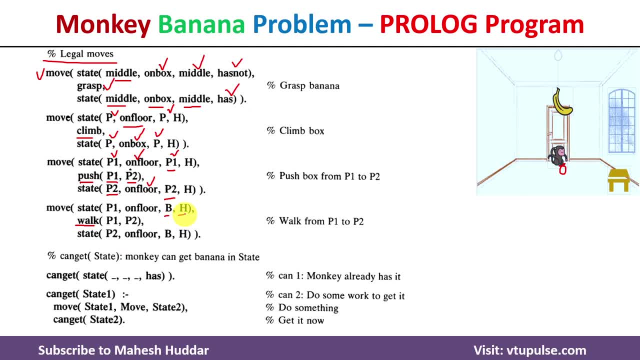 we don't care about the box and the monkey is having banana or not. We care only about the initial position and the monkey is present on floor or not. These are the only two things we will see Whenever it executes a walk from P1 to P2, it will go from P1 to P2 and still it is present on the floor here. So these are the 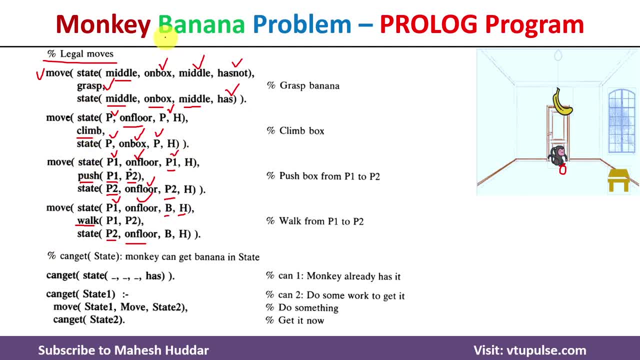 four legal moves in this monkey and banana problem here. Now the next thing is: there is one very important thing. There is something called as a termination condition. here We will check the current state, whether the monkey is having banana or not, To check that particular thing. 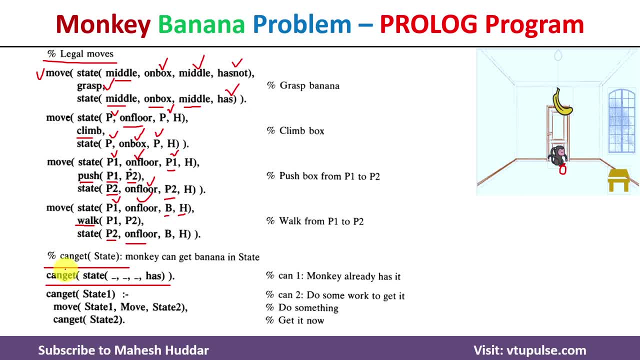 what we do. We execute this particular command, that is, can get state. We don't care about the first three components, We care only about the last component, whether the monkey is having banana or it is not having banana here. So that's the reason, the last component, we have written here. 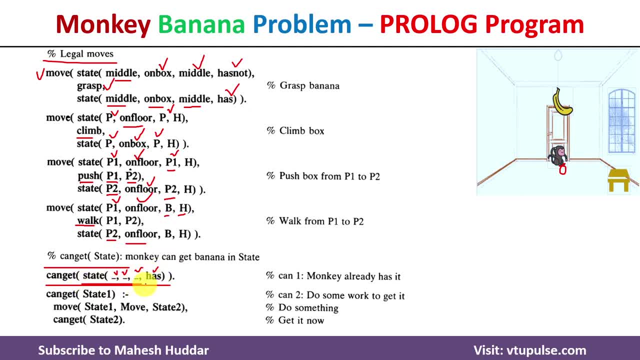 has here. So whenever monkey has the banana, this entire thing will be written new. The true here. the meaning is: monkey got the banana. We will stop over there until it becomes has. We have to execute these legal moves again and again, in this case Now, at the initial stage. 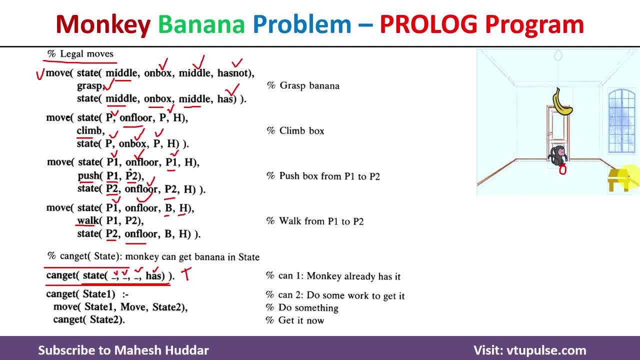 the monkey is present at door box, is present at window and banana is hanging exactly middle of this room. The meaning of this one is: monkey is not having banana, So because of that, this can get. state 1 will return false here. Because of that, we need to execute the possible. 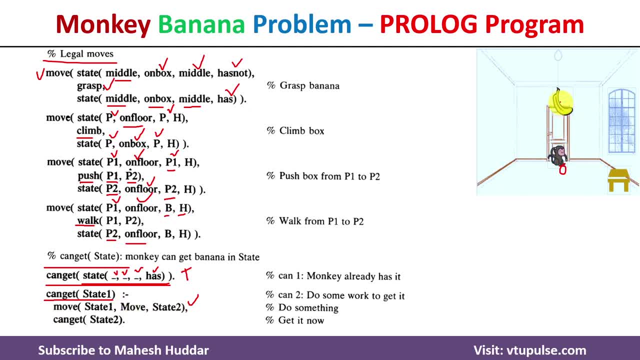 moves again and again until the monkey gets these bananas in this case. So that's the reason we need to execute the legal moves, one after the other, until the monkey gets these bananas in this case. So what we do here is we will check the initial state. What is the 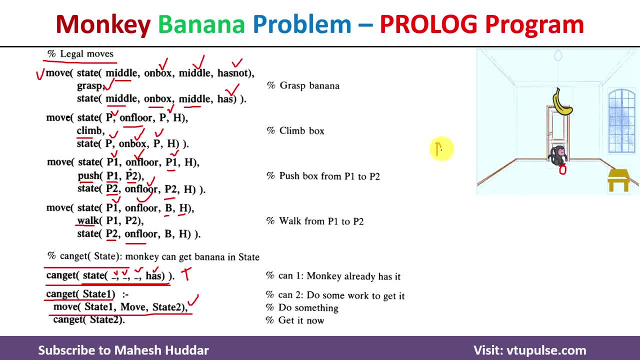 initial state: Monkey is present at door here, It is present on floor, The box is present at window and it is not having banana, not having banana at this particular thing. Now we will check it out Out of these particular four possible moves which will match here Now, the 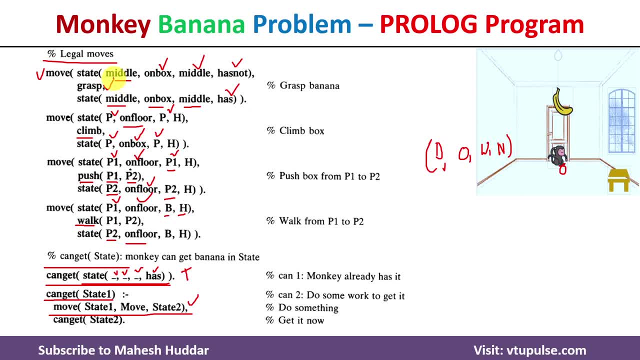 first one will not match because this will be executed only when the monkey is present at the middle. Again, it will not be executed. Second one: both monkey and box should be present at the same position, But in this case monkey is present at door and box is present at window. So second one: 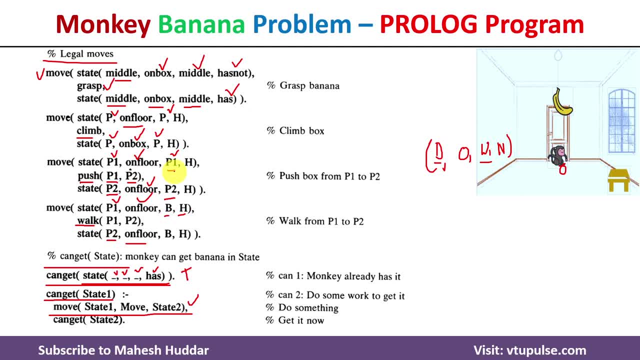 will not work. Third one: monkey and box should be present at the same position. Then only we can execute push here. The fourth move is: monkey is present at P1 position. That is nothing but door. We don't care about the box here. So 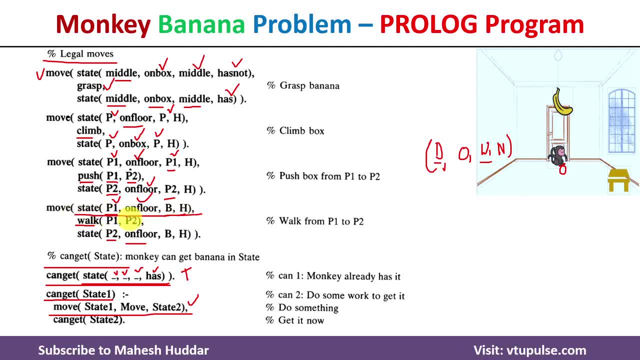 this is perfectly a valid move in this case. So once we execute this walk move, the monkey will go from P1 to P2.. So P1 is what? in this case, P1 is at door. P2 will be nothing but what. 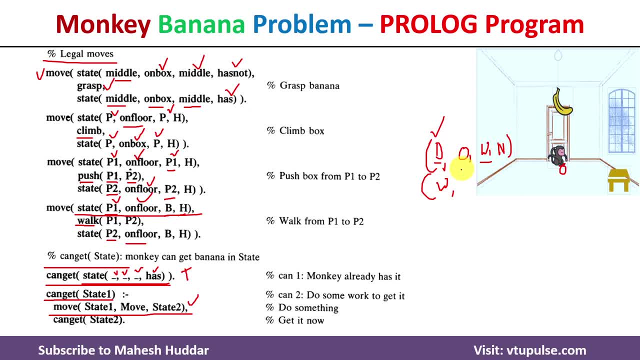 Window here. That is what the thing will happen. It will go to window on floor. only The box is present at window and monkey is not having banana. This is what will be the current state now. Now, once it comes to this current state again, we will check whether the monkey got the banana. 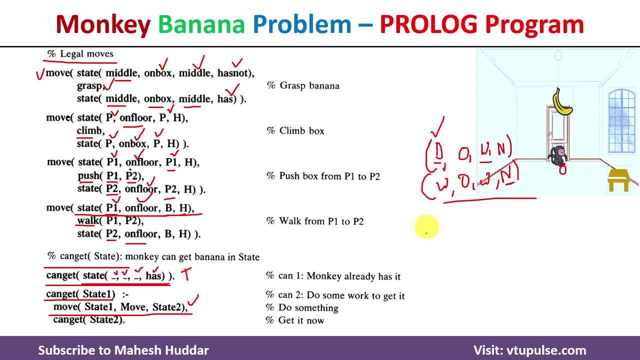 and can get straight to. Right now it has not got the banana Again. it will go back and then it will execute one more move here. Now, whenever it wants to execute move again, we need to check it out. The monkey is present at window and box is present window here. So first one will not match. 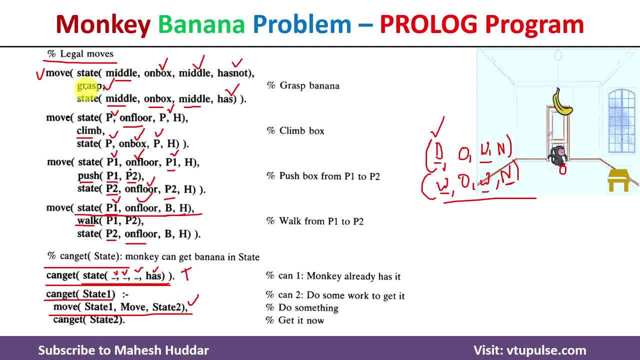 because monkey should be present at the middle. Then only we can execute grasp here. So it will go to this one, That is, monkey and box are present at the same position, that is, P and P. But what we are expecting is monkey should be present at the middle. So here it will go to this one, That is. 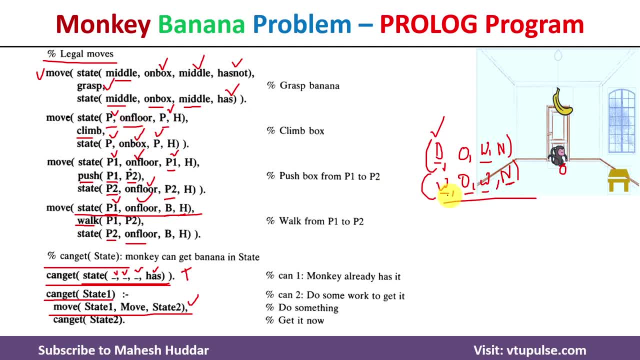 be present on floor again. that is also satisfied. here now, all three things are satisfied. the meaning is this: claim: boom will be executed. after that, what will happen? uh, it will move to the same position. that is a window. it will go to on box here. it will go on the top of box here. window. 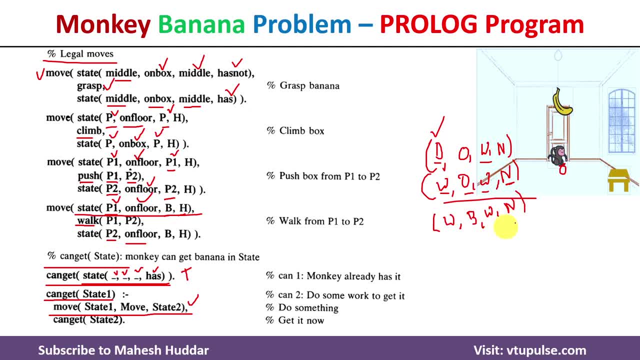 and still it is not having banana in this case. now, if you look at these things, uh, after executing the second one, still it has not got the banana again. the next move will be executed. both monkey and box are present at the same position now it is present on the top of box here. 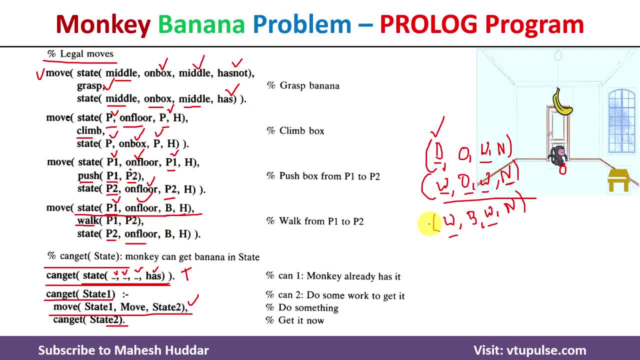 none of these things will match here. because of that, we have to backtrack to the previous state here. so this is what the previous state here. now, when you go to the previous state rather than executing claim, do you have any other moves? we have to check it out. 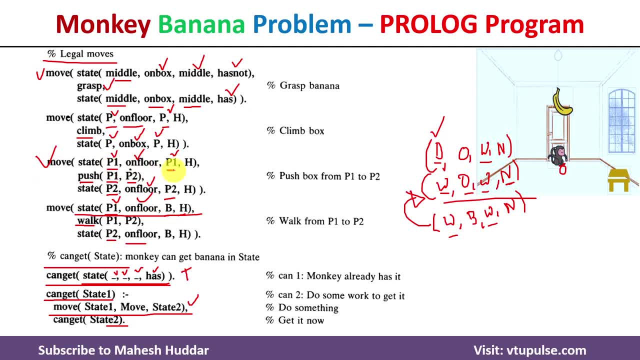 now, if you look at this particular move, both should be present at the same portion, that is, monkey and box, and we are expecting monkey should be on the floor again. it will match here. so what we can execute is: we can execute push here, the monkey will push the. 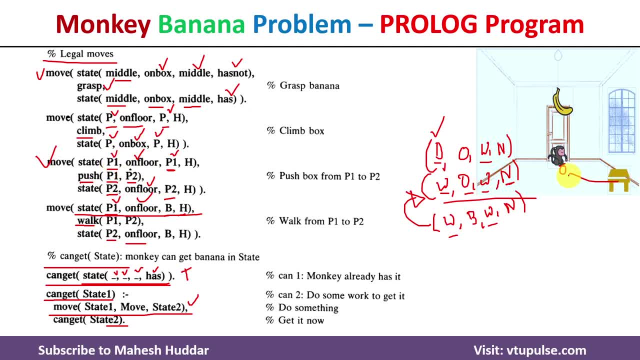 box from p1 to p2. here the meaning is it will go from here to here. the box will be present exactly at the center now. now what will happen? so it will go to a middle here and then it is present where it is present on floor and then, where it will move again, it will be present at the middle. still, it 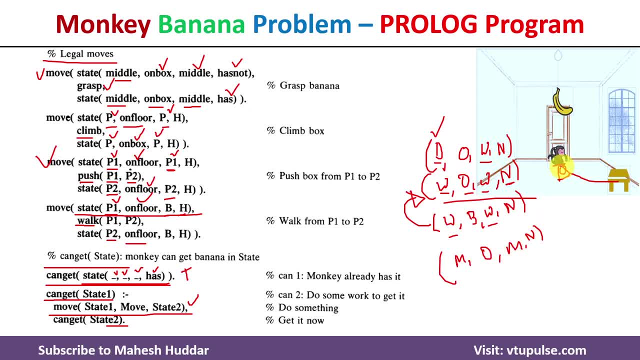 has not got the bananas. in this case. now the monkey is present at the middle, box is present at the middle, but monkey is present on the floor here now. still it has not got the banana. we have to execute the next move. the next move: we have to check any of these things middle, middle, of course. 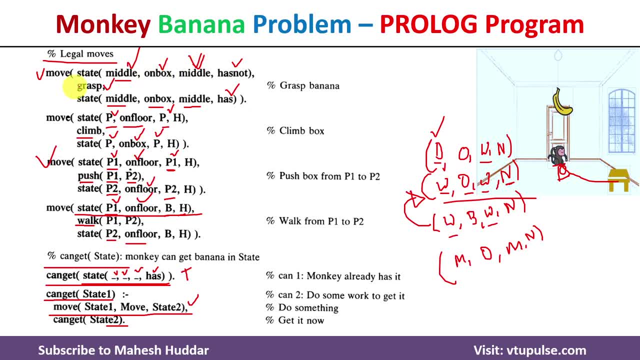 both these things will match here, but what we are expecting for grasp, we are expecting monkey should be present on the box here. so this will not match, so we will go to the next one. monkey and the box are present at the same position, that is, p and p. in this case it is. 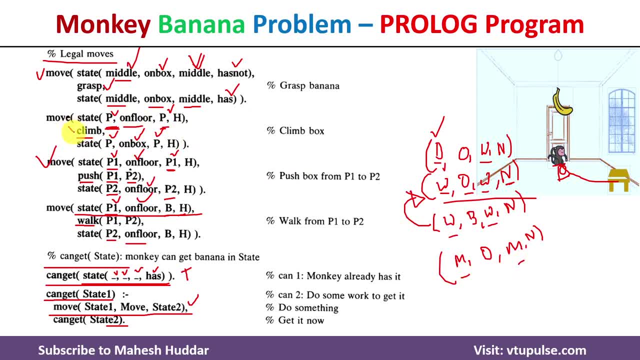 middle and middle. uh, it is present on floor. so what we can execute here clip, we can execute one. once we execute the claim, it will be present at the same position. that is middle and middle. but what will happen is the monkey will sit on the top of box here. 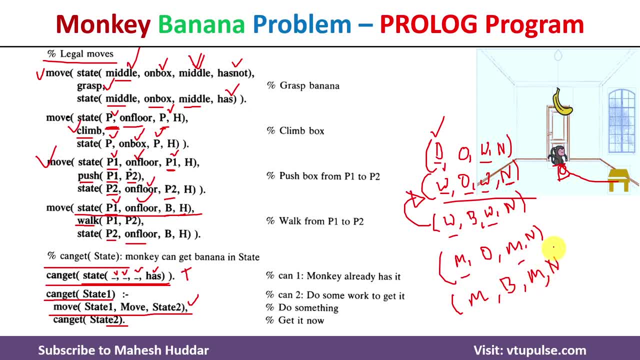 it is nothing but b in this case, and still it has not got the bananas in this case. so this is what we have executed. again, we will check whether we have reached that target or the goal. uh, still we haven't reached the target because we are expecting, as here. so we will. 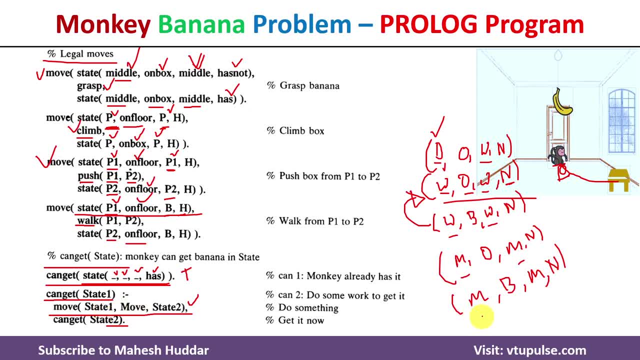 go back and then execute one more move. in this case, uh, once you look at this one middle on the top of box, middle and not- this will exactly match the to this particular initial state here. so what will be executed now? grasp will be executed. once you execute the grasp, it will become middle on. 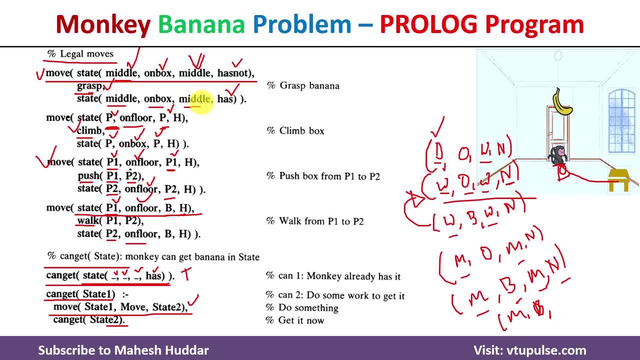 again. it will be on box that is b only. uh, this one will be middle again. and then what is the last component? previous it was not. now it has has that particular banana. so because the banana is present once you execute, this can get for the state 2. 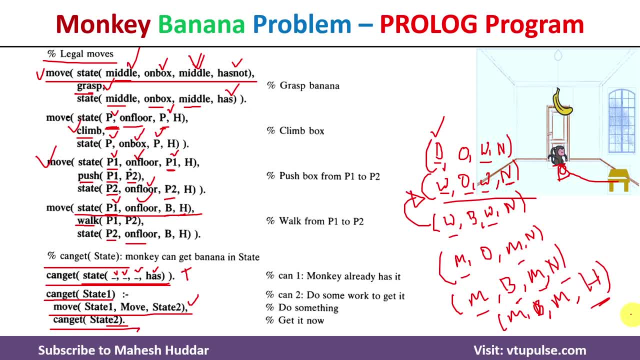 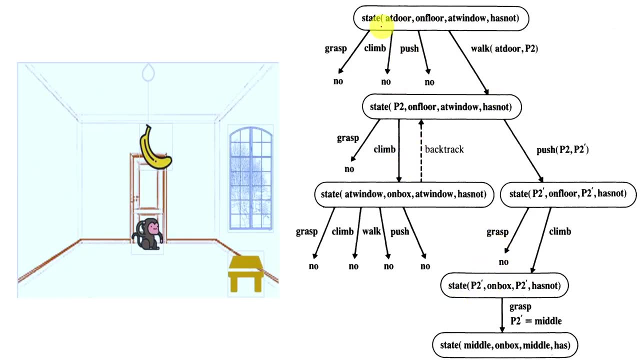 it will return you. true, the meaning is: the monkey got the banana in this case. so the execution will stop in this case. so it will start from the initial state. it will go from one state to other state until it will reach this particular goal state. the same thing has been shown in this diagram also. 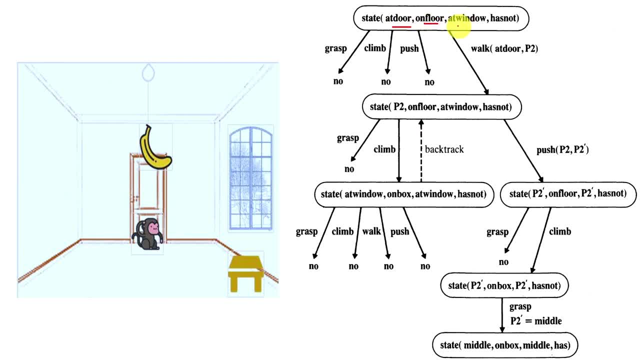 initially. the monkey is present, at door, on floor, at window box is present. the monkey does not have banana. so what are the four possible moves are there: grasp, climb, push and walk. these three are possible. that is what i have explained in the previous program. only walk is possible, so it will. 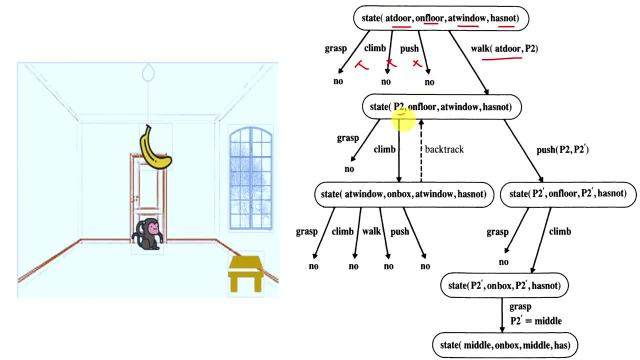 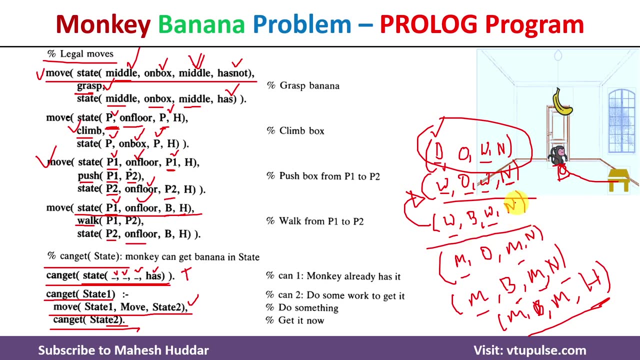 go from at door to p2. here the p2 is nothing but one at a window. in this case, at this particular position, again, we have four possibilities out of that. grasp cannot be executed, claim can be executed. that is what we have seen here. we have executed claim we want. we got to this particular 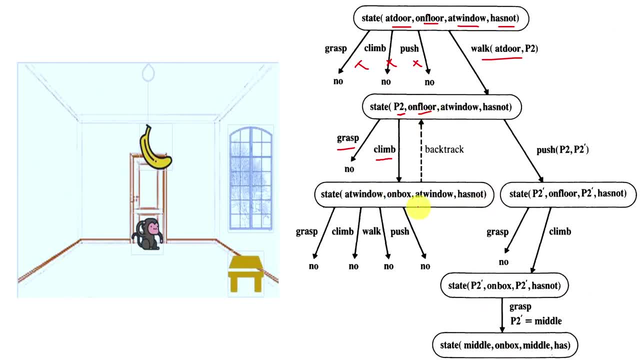 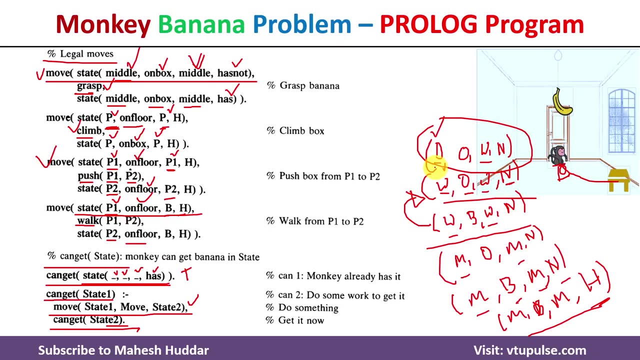 state here. that is nothing but from on floor. it has got to where it has got to on box here that we need to go to the previous state. but when you go to this on box, that is after this claim, we cannot execute any of the moves here. so that's the reason what we need to do. we need to backtrack. 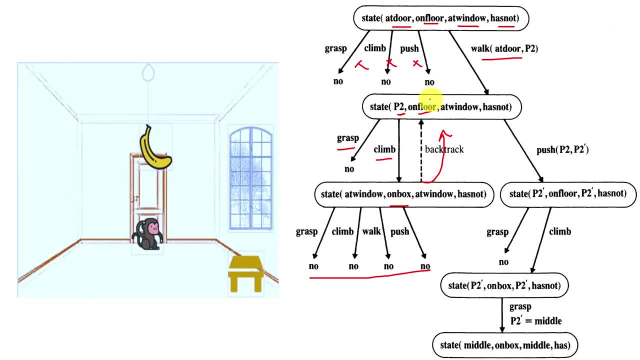 here. that is what i have explained here. also, we have to backtrack to the previous state. now, once you go back to this previous state, what we need to do we have to execute any other moves possible at this particular state. we have a move possible that is called as push in this case. so what will? 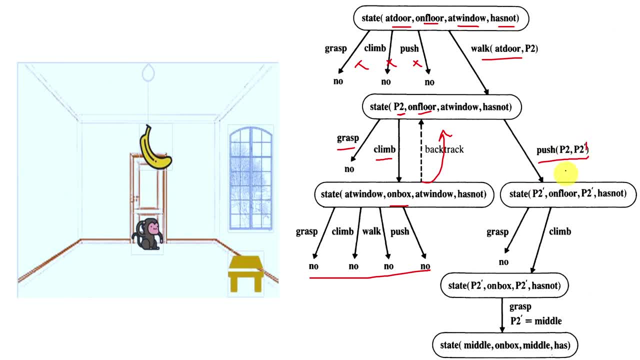 happen, the box will be moved from p2 to p2 dash. in this case, p2 dash is nothing but a push. we will try to do some about what middle in this case. so it will be moved to, uh, p2 dash. that is nothing but a middle. 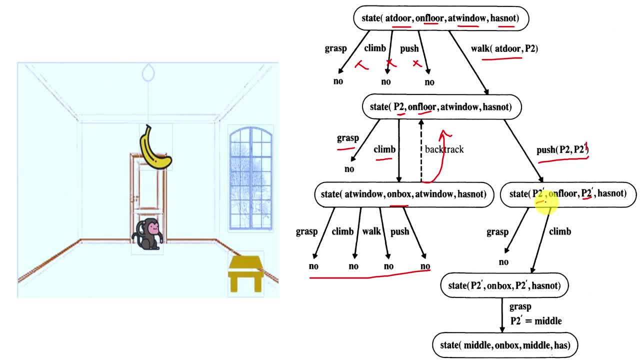 uh box is present at p2 dash and monkey is also present at the p2 dash. here again, grasp cannot be executed. we can execute claim. this on floor will become what on box. that is what i have shown here on floor will become what on box in this case. now, once it is present on the box, uh, p2 dash and. 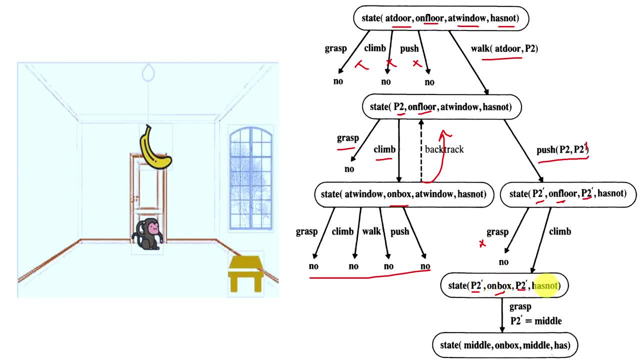 p2 dash is nothing but middle here, middle on box. middle has not. grasp will be executed. what will happen? it will be present at the middle, only on box. but the monkey got the banana. that's the reason this has not is changed to as in this case. so because we got has at the last component of 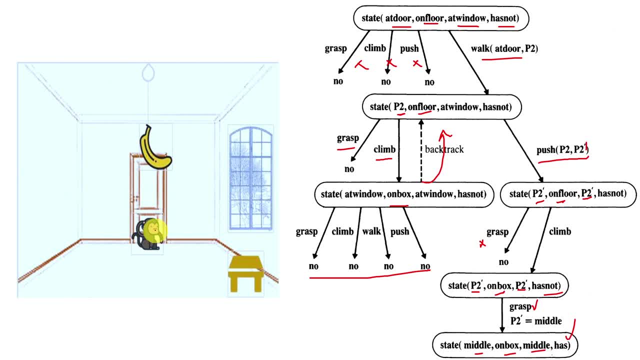 the state here. we will stop here. the meaning of this one is: monkey has got the banana at this particular position. in this video i have discussed how can we write a program to solve monkey banana problem in prologue programming language. in the previous video i have discussed 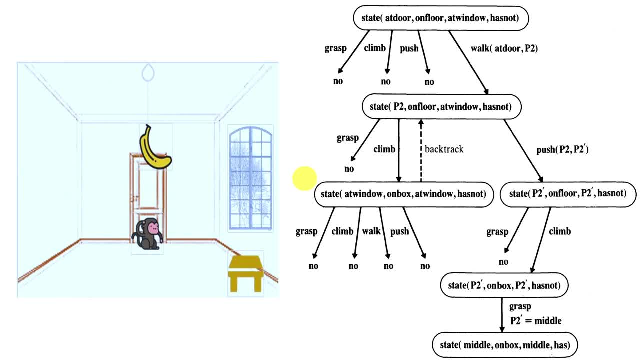 the basic concept of monkey banana problem, that is, how to define a state and how to define a moments. link for that video is given in the description below. i hope the concept of monkey banana problem is clear. if you like the video, do like and share with your friends. press the.